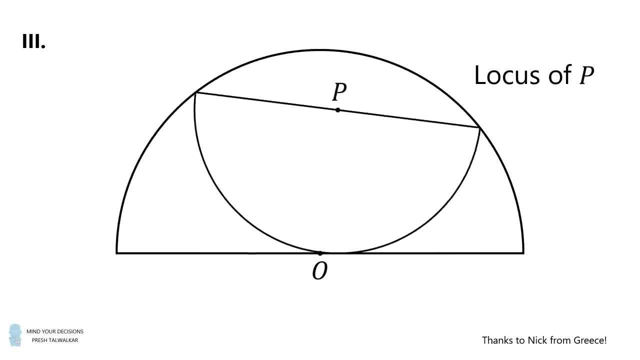 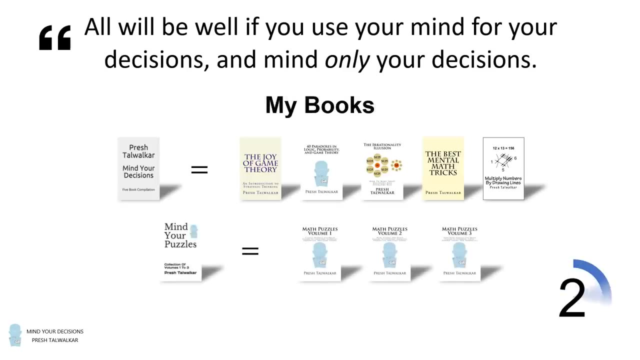 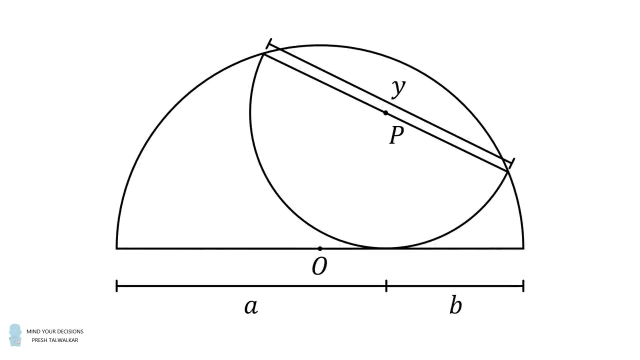 Pause the video if you'd like to give this problem a try and, when you're ready, keep watching to learn how to solve this problem. Let's solve for the general case first. Let T be the point of tangency along the large semicircle's diameter and let Q be this upper point of tangency. 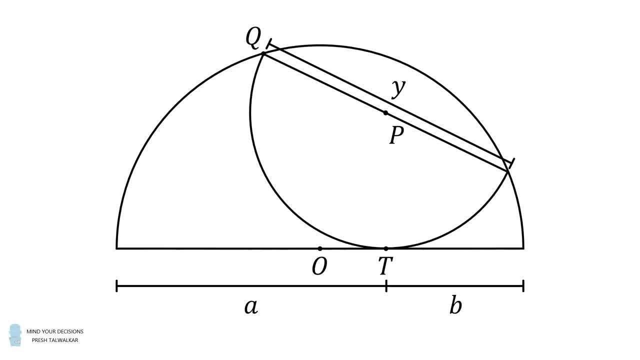 Since the inscribed semicircle has a diameter equal to y, its radius will be equal to y over 2.. Construct the radius PT, Because T is a point of tangency. PT will be perpendicular to the diameter of the large semicircle. 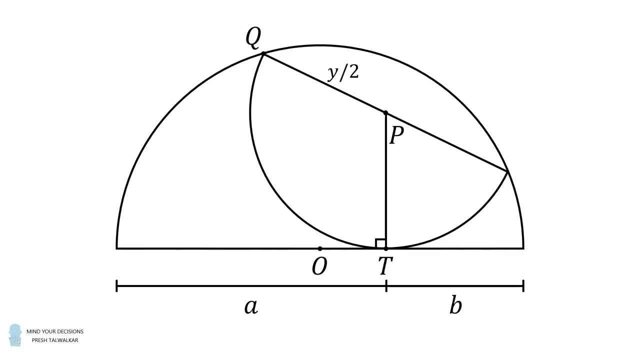 Furthermore, it's a radius of the inscribed semicircle, so its length will be equal to y over 2.. Now construct OQ. It's a radius of the large semicircle. The large semicircle has a diameter equal to a plus b, so its radius will be half of a plus b. 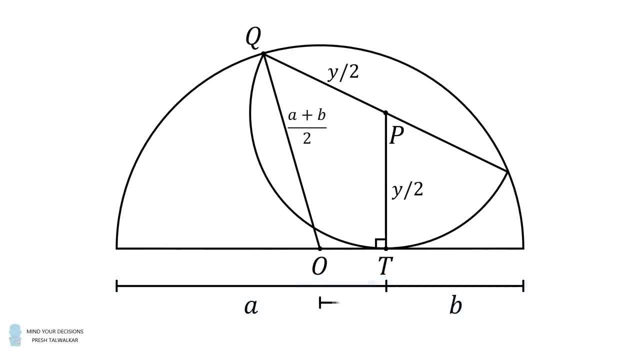 Next construct the distance, OT. Its distance will be equal to the radius of the large semicircle minus b. We can substitute for the radius of the large semicircle and then we can simplify. OT will be equal to a minus b, all over 2.. 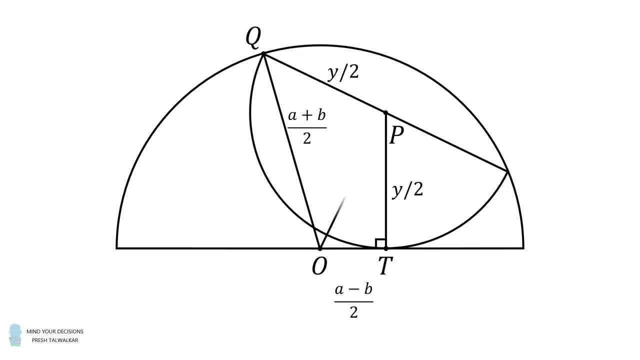 Now construct the radius that goes through the points O and P, Because this bisects the diameter of the inscribed semicircle. it will be the perpendicular bisector. We now have two different right triangles that we can focus on. Let's get rid of everything else. 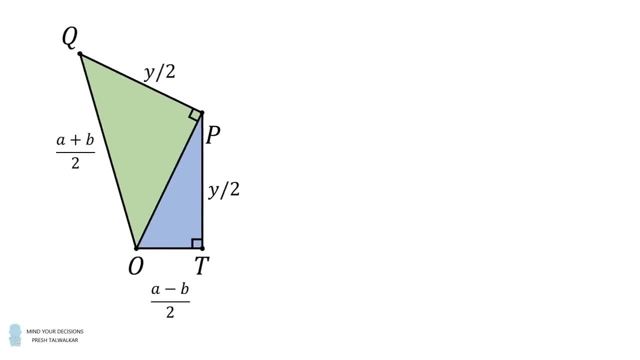 We will now calculate the length OP squared in two different ways. First, let's calculate it in the blue triangle. It will be equal to the quantity a minus b, all over 2 squared, plus a minus b, all over 2 squared plus y over 2: the quantity squared. 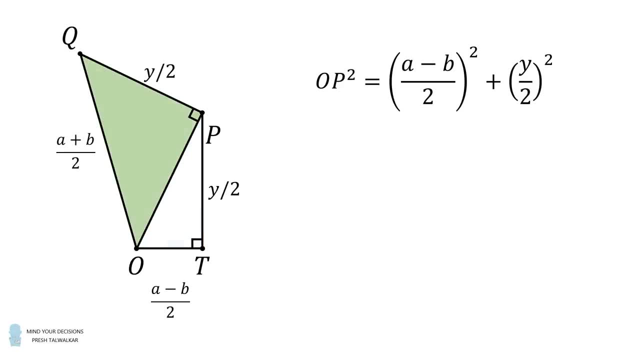 Now in the green triangle we can calculate op squared in a different way. It will be equal to the square of the hypotenuse of this triangle minus the square of one of its legs. So this will be the quantity a plus b over 2 squared, minus y over 2, the quantity squared. 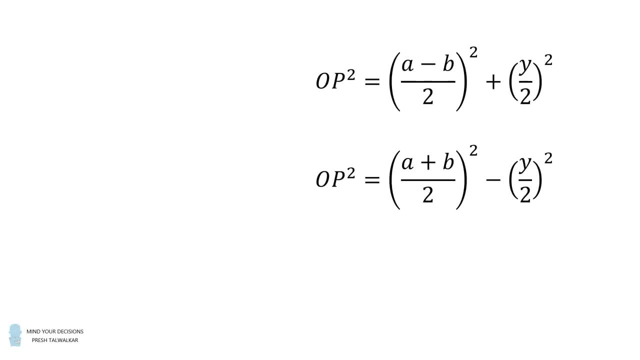 We have two equations that are equal to op squared, so we can set these two equations equal to each other. Let's do that. We will now simplify by squaring each term. Now, each term has a denominator equal to 4, so these will cancel out. 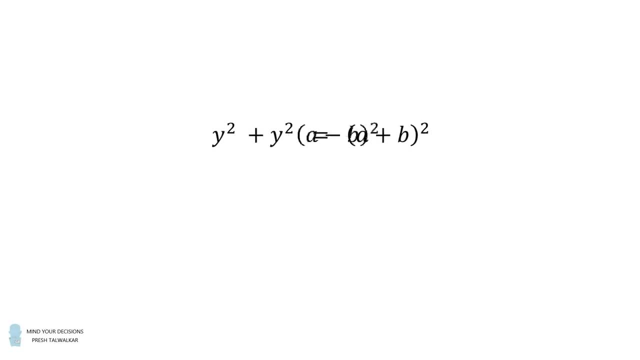 We will now group like terms. We will then simplify this equation. The left hand side is 2y squared, and the right hand side will expand each binomial. We can then cancel out a squared, So we are left with: 2y squared is equal to 4ab. 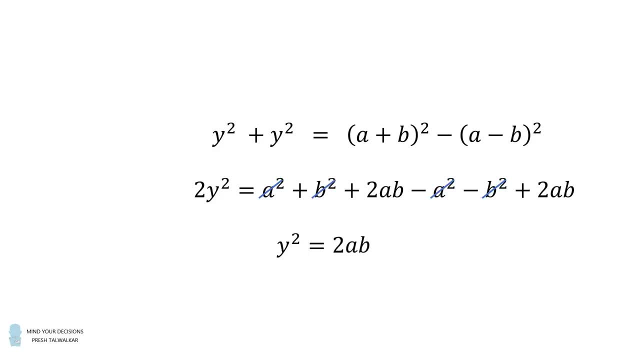 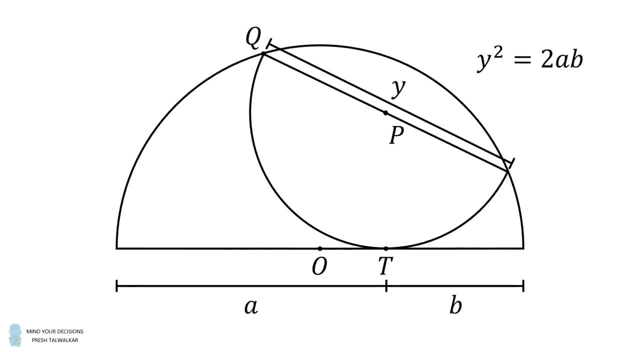 We divide both sides by 2, and then we simplify. Thus y squared is equal to 2ab. So we solve part 2 of the problem. We have y as a function of a and b. If we wanted to be more explicit, we could say: y is equal to the positive square root. 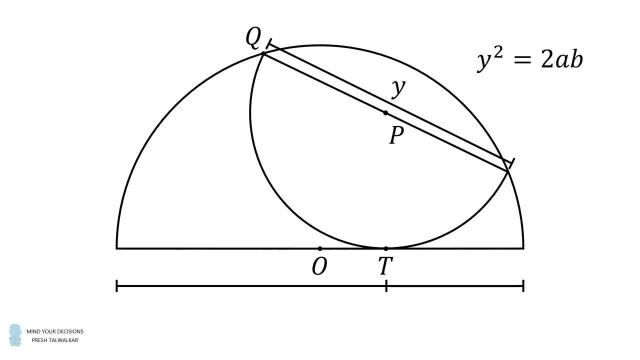 of 2ab. Now let's tackle part 1.. We have the two distances: a is equal to 2, and b is equal to 1.. So we substitute y: squared is equal to 2 times 2 times 1.. 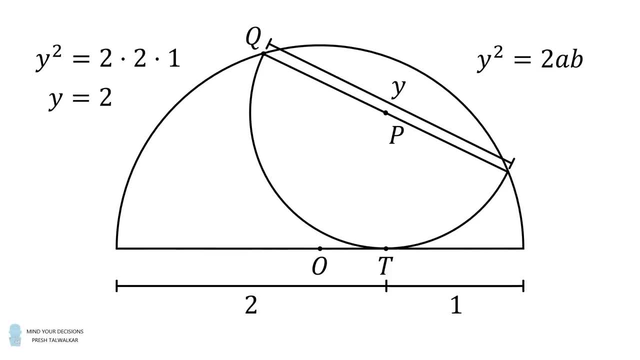 This means y squared is equal to 4, and y is equal to 2.. That's part 1 of the question. Let's now tackle part 3.. Consider the triangle OTP. We know that pt is equal to y over 2.. 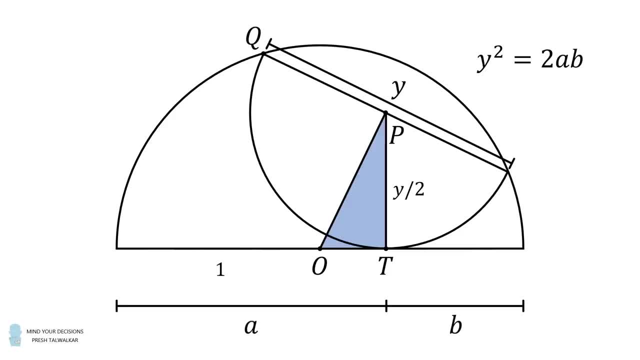 Without loss of generality. suppose the large semicircle has a triangle. We know that pt is equal to y over 2.. The small semicircle has a radius equal to 1. Suppose that ot has a length equal to x. 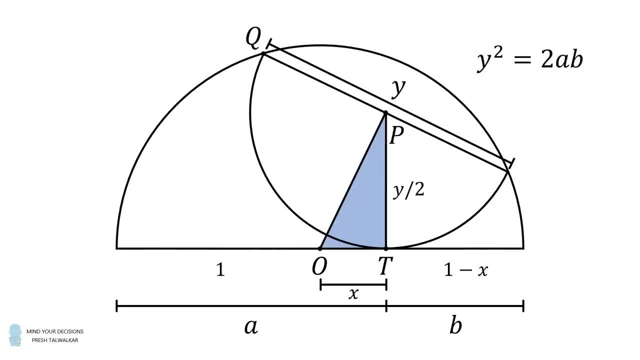 Then the remaining distance will be equal to 1 minus x. From our formula that y squared is equal to 2 times a times b, we can see that a here is equal to 1 plus x and b is equal to 1 minus x. 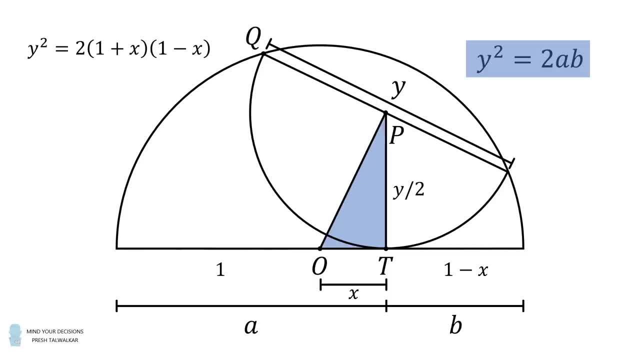 So we have: y squared is equal to 2 multiplied by the quantity 1 plus x multiplied by the quantity 1 minus x. We can simplify this: y squared is equal to 2 minus 2x squared. Now we're interested in the locus of point P.